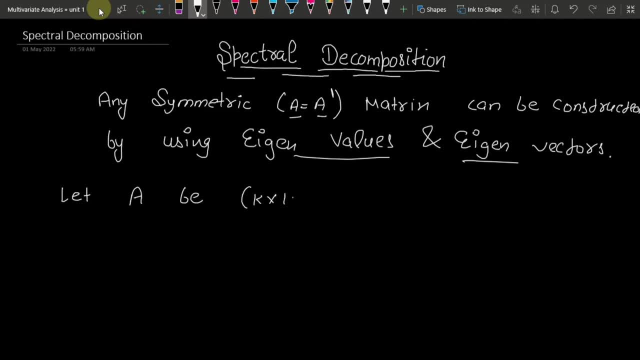 square matrix. K by K is a square matrix, K by K is a square, symmetric matrix. So what can we do now? And we know that the order of the matrix K by K is equal to its eigenvalues, So A is also K by K square matrix, having K non-zero eigenvalues. K have non-zero eigenvalues. 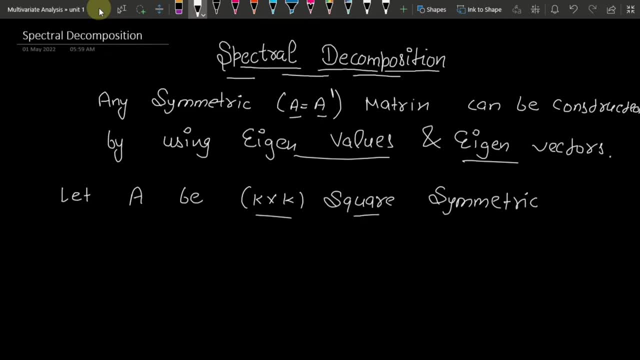 having K eigenvalues. So let's assume that the eigenvalues of K are. what are those? We denote eigenvalues from lambda, So lambda1, lambda2 up to lambda, So we can define them all with a first person window of lambda, So lambda1, lambda2 and lambda2 out to lambda. 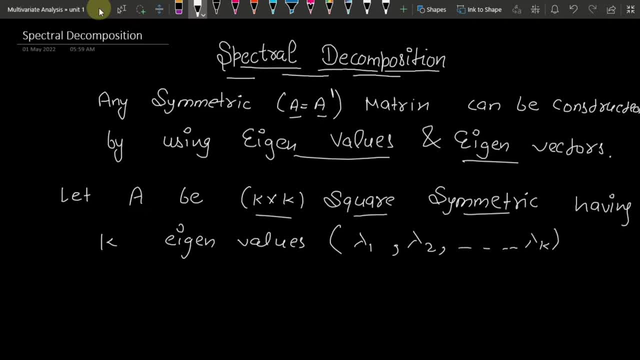 treats the values of K by K. Note that in MLA, same as in PHP, make a dependency Methods. So K is the eigenvalues with eigenvectors. So we had studied the normalized eigenvector. So what is the normalized eigenvector of the matrix? 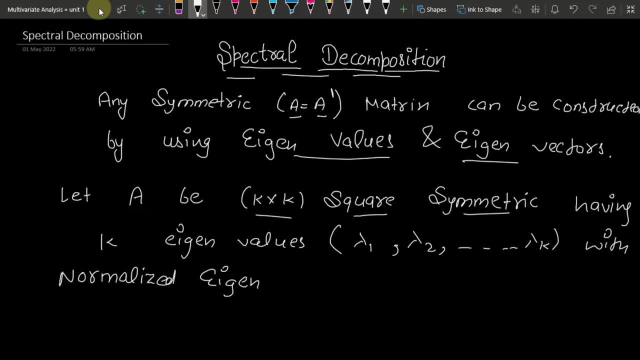 With normalized eigenvector. As we know, every eigenvalue, ie every lambda's possible value, has an eigenvector. And what is the normalized eigenvector? If we divide the original eigenvector by its length, then it is a normalized eigenvector. 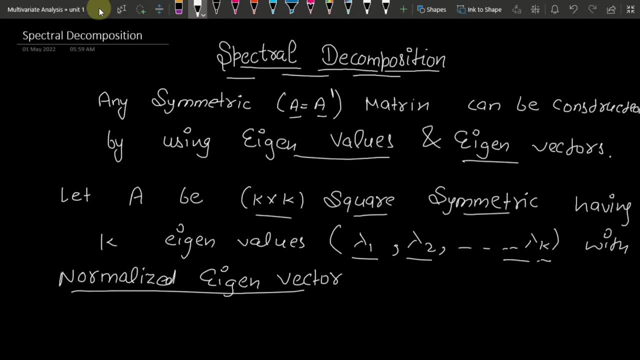 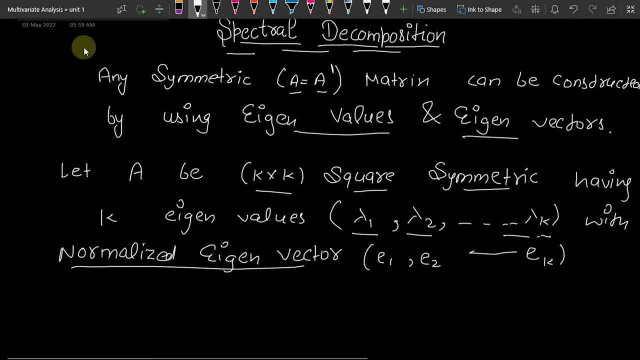 Which we denote by EI. So here we have E1,, E2, all the eigenvalues of lambda, K, E, which will be the eigenvectors. So we have taken a matrix, a square matrix, So here we can construct A. 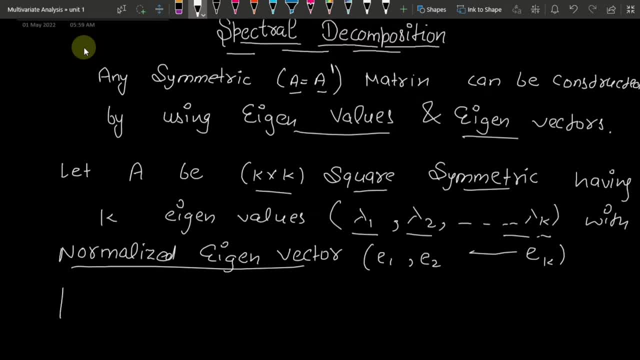 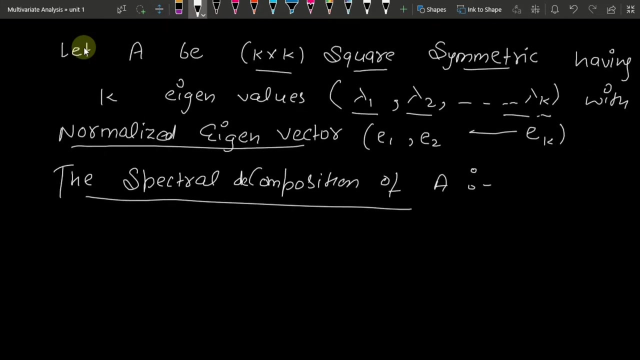 So its spectral decomposition will be A, So the spectral decomposition of A, The spectral decomposition of A, So the spectral decomposition of A, is given by E1, E1. transpose lambda 2, E2, E3, E4, E5, E6, E7, E8, E9, E10, E11, E11, E12, E12, E13, E14, E15, E15, E16,, E17,, E18, E19, E19,, E20,, E21, E21, E22, E23,, E24, E25, E25, E26,, E26, E27,, E28,, E29, E29, E30, E30, E31, E31, E32, E33, E33, E34,, E34,, E35, E35, E36, E36, E36, E37, E37, E38, E38, E39, E39,, E40,, E40, E41, E42,, E42,, E43, E44, E44, E44, E44, E44, E45. 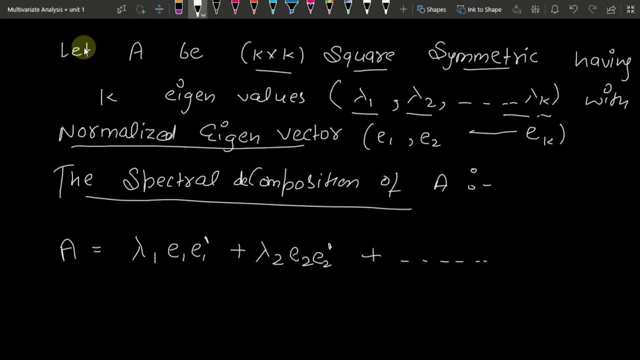 E42, E2 transpose, then plus up to jitne eigen value hai, then jitna os matrix ka order hai, uthne hi eigen values. tak ye spectral decomposition hum write kar rahe hai. So spectral decomposition ka matlab hai, ki humne ek matrix ko decompose kar diya, means humne usko uske eigen values aur eigen vectors ki form me usko represent kara hai. 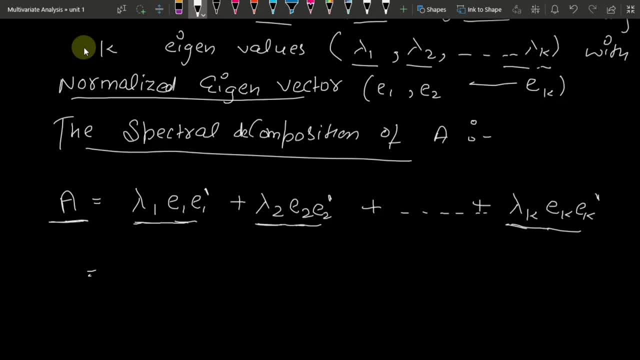 So agar hum isko combine kar ke likhen, to kya likha jayega: sum ho rahe hai, summation hai. so hum yaha par summation laga denge, jaha par i ki value rahe ge wo 1 se lekar. kaha tak rahe ge kyunki: lambda 1, E1, E1 transpose. lambda 2, E2, E2 transpose, then lambda k Ek Ek transpose. 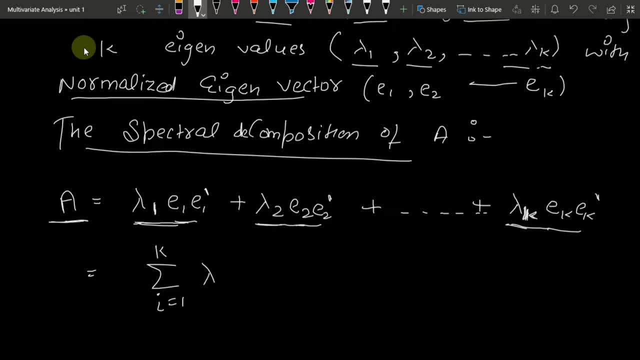 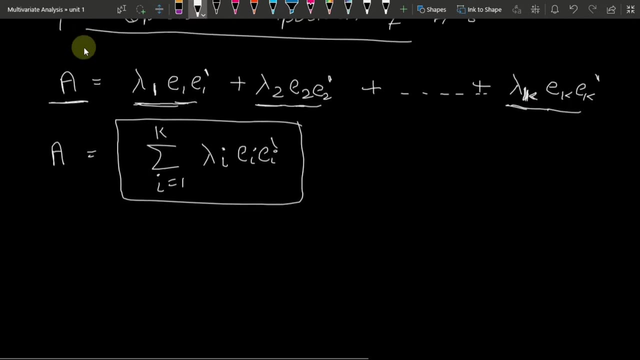 So i ki value 1 se lekar k tak ja rahe hai to hum yaha likh denge lambda i Ei Ei transpose. So yeh apke paas is tarike se general formula rahe raha. spectral decomposition ka means, aap kisse bhi matrix ko uske eigen values, eigen vectors ki form me represent kar sakte hai. 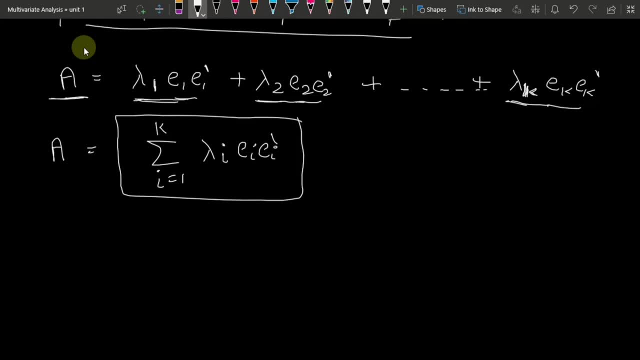 Means, agar aapko koi bhi matrix ke eigen values aur eigen vectors dahi rakhe hai, to aap unka use karke matrix ko find out kar sakte hai. Abhi tak to aap matrix ko use karke eigen values, eigen vectors find out kar rehte hai, but aap jo eigen values aur vectors hai, unki health se matrix ko construct bhi kar sakte hai. 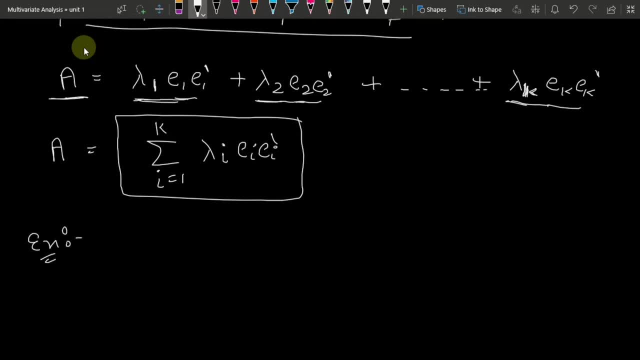 Ek example. dekhte hai, kaise hume karna hai, ishe iska proof. dekhte hai, kya actually me koi bhi matrix uski eigen values aur vectors se construct ki ja sakte hai. So dekhiye, agar aapke paas ek matrix de rakhi hai, 1,, 2,, 2, minus 2, to hume iska find out the spectral decomposition. 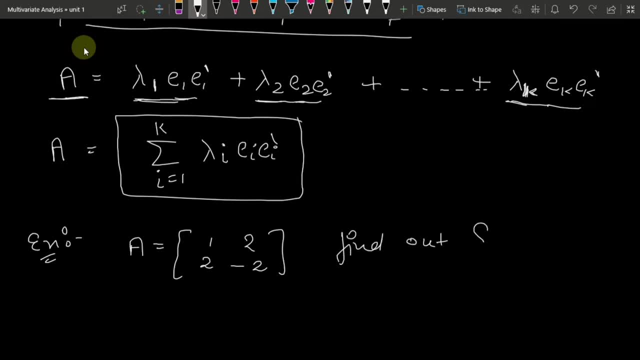 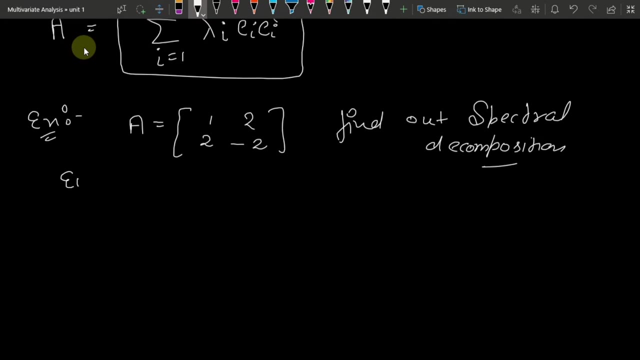 To hume iska spectral decomposition kar sakte hai. find out the spectral decomposition. so first of all we have to find the eigenvector. so we know what we use to find the eigenvalues. in the last video we studied to find the eigenvalues we use the characteristic equation and that characteristic equation. 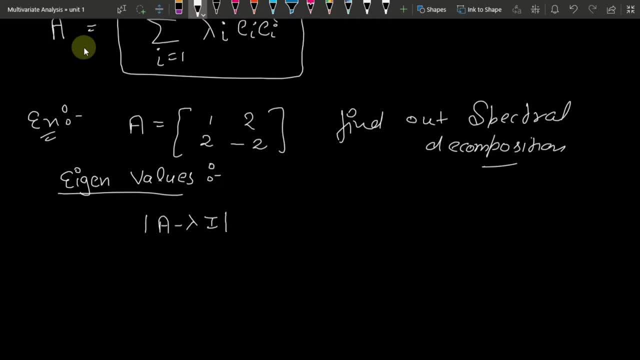 we have a minus lambda i, the determinant equal to zero. so here what we will do when we put a in place of a. so here it will come one, two, two minus two, and then after this minus lambda i, so i will take the order of a matrix will remain the same as the order of identity matrix. 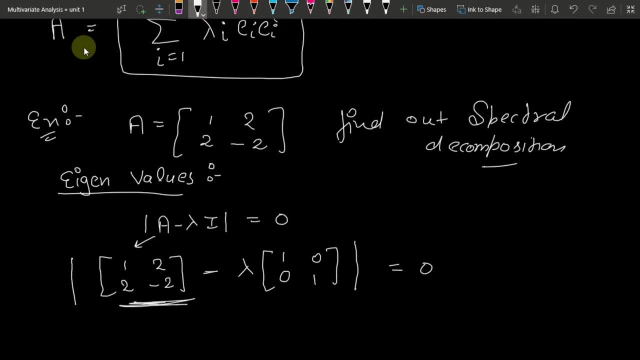 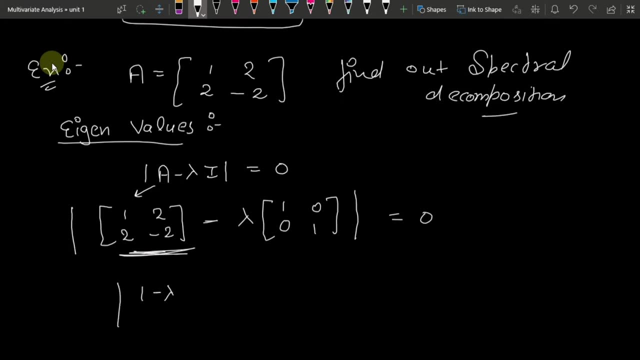 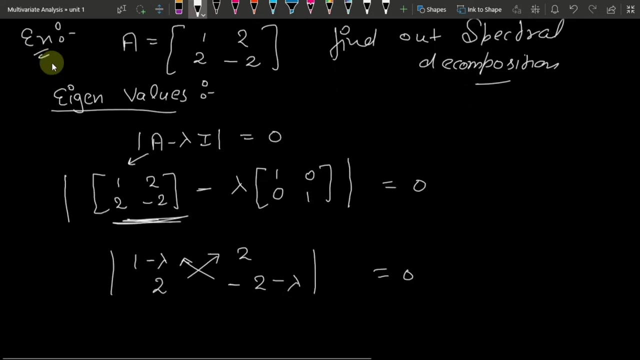 so in this way we will equate it with zero. so when we solve it here, so after solving, we will get the necessary direct, some média of of two to two minus two minus two minus lambda. so when you solve this determinant, do you know, in the case of two by two order, we do it through cross multiplication. 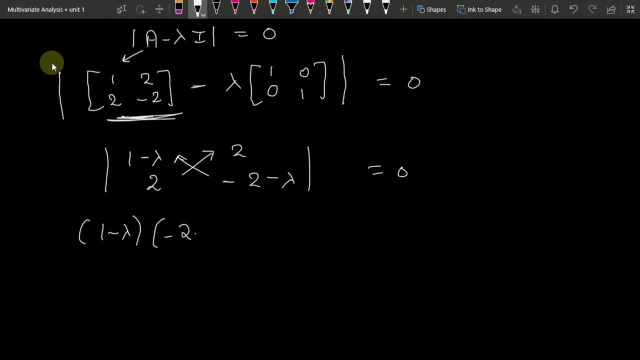 so here, when we do cross multiplication, then this will be equal to one minus lambda multiplied minus two minus lambda, minus two to the four is equal to zero. so when we solve this, this can be plus or minus two or minus lambda, lambda plus 2, lambda plus lambda, square minus 4 equal to 0.. So from here we will get a quadratic. 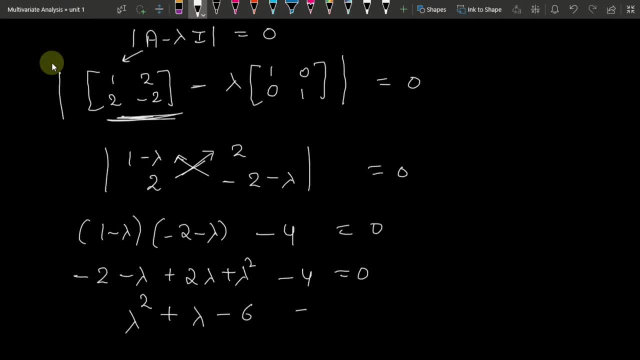 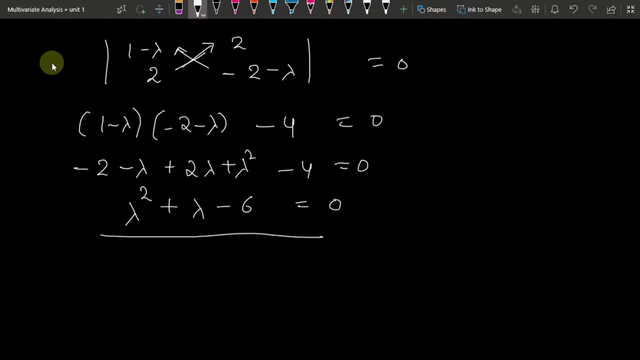 equation: lambda square plus lambda minus 6, equal to 0.. So now you will tell us the factors that we got the quadratic equation because the order of the matrix was 2 by 2.. So here we will get a quadratic equation where we will get two roots and those two roots will 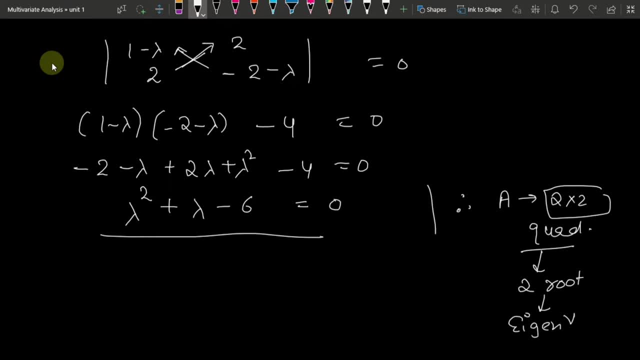 be our eigenvalues. So here, when we solve this, we will get the factors that we got. the multiplication should be minus 6, but plus minus should be plus 1.. So here we will take plus 3 lambda minus 2, lambda minus 6, equal to 0. So when we solve this, we will get the 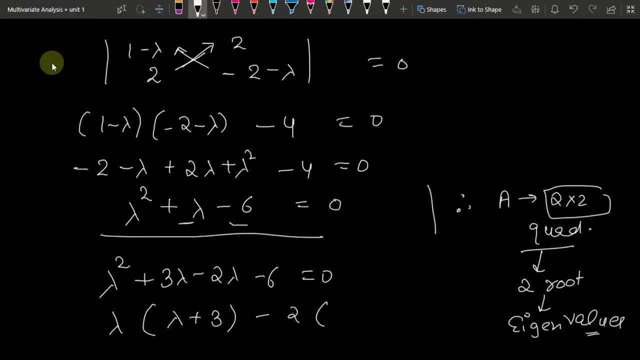 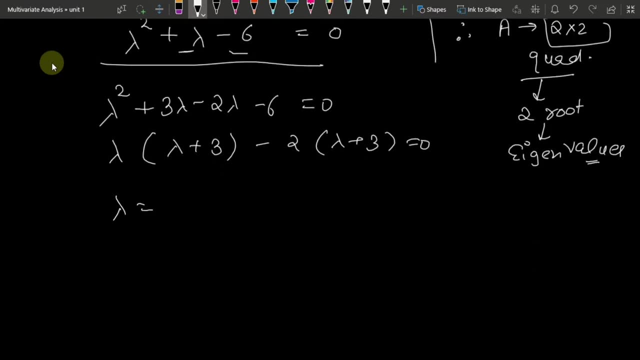 lambda. common here: lambda plus 3 minus 2. common here: lambda plus 3.. So from here the possible eigenvalues will come. here lambda is equal to, so lambda 1 means first eigenvalue will be minus 3 and the second eigenvalue that we have that is equal to lambda 2 will come. 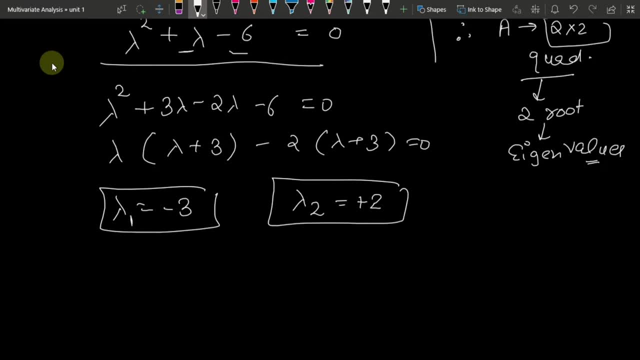 here plus 2.. So how much is lambda 2 plus 2? because here lambda minus 2 equal to 0. so lambda 2 equal to plus 2.. So here you have two eigenvalues. These two eigenvalues will be given, and by using these two eigenvalues you have to find out its corresponding eigenvectors. 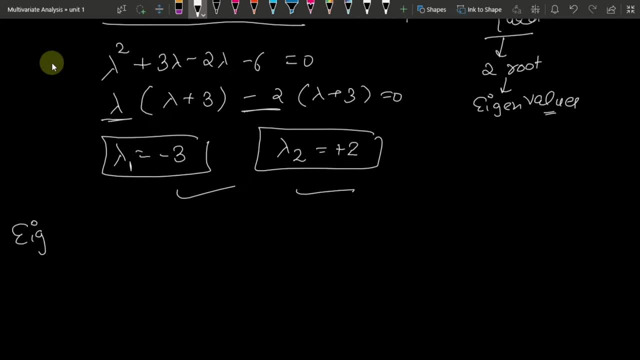 So we have found out the eigenvalues. Now we will find the eigenvectors. So now the eigenvectors. So how do we find out the eigenvectors Corresponding to each eigenvalue? which means: since lambda is 1, the corresponding eigenvector will be x1.. Since lambda is 2, then the corresponding. 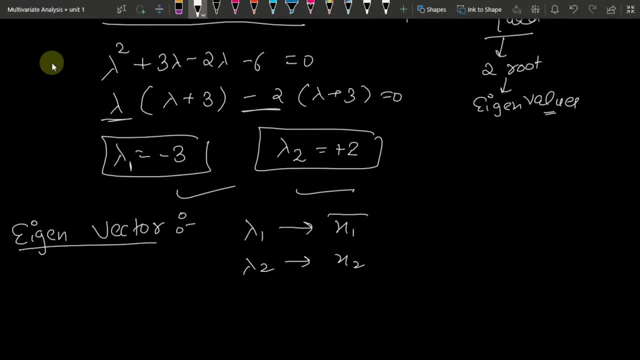 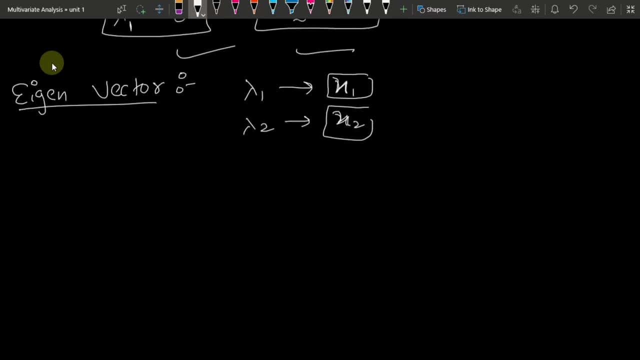 eigenvector will be x2.. So now we have to find out x1 and x2. only we have to find out. we have to find out these vectors. so to find them out, what equation we had we used to use? equation a into xi is equal to. 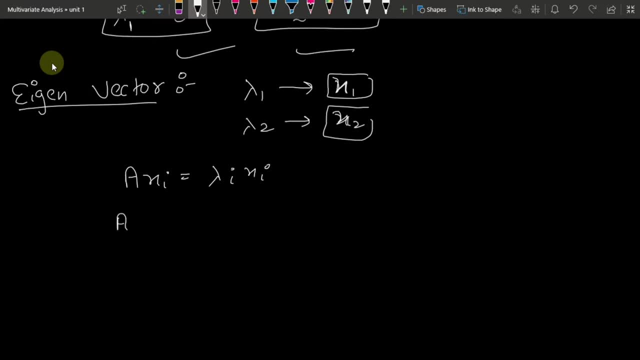 lambda i, xi. so here a, as it is xi. first of all we will find out xi because where will our value of i go from 1 to 2? because we have 2 eigen values. so here xi is equal to lambda 1. xi means first of all how much we put xi. 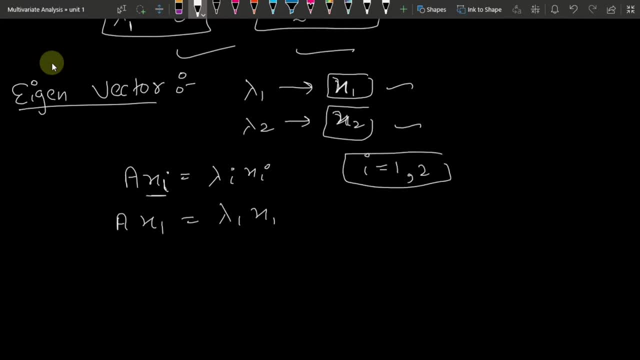 1 foot or 2 foot. so here, what is the value of a? we have 1, 2, 2 minus root. because our matrix is given, that is a and here x1. we have to take x1 in such a way that the order of matrix is 2 by 2. 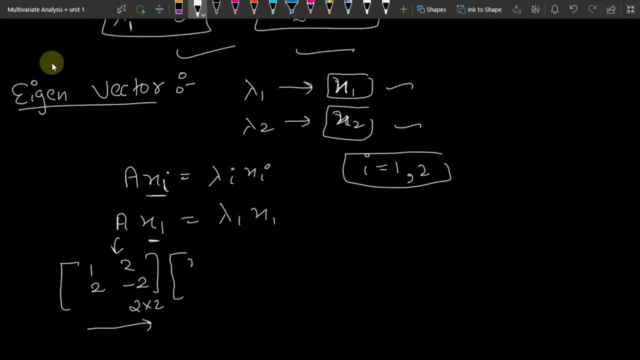 so the multiplication will be possible. so we will take x1, 1, x1, 2. in this way its order will be 2 by 1, because how many columns are there in a vector 1 and how many rows can be there. so if there are 2 columns, 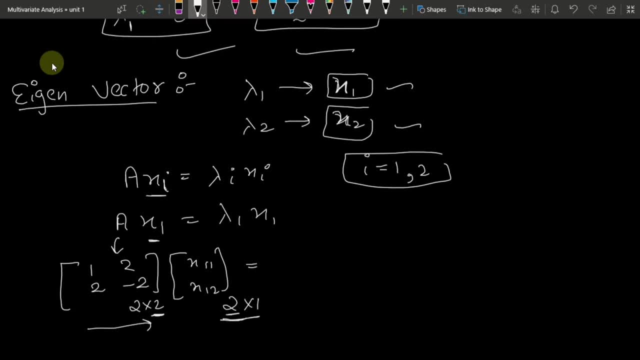 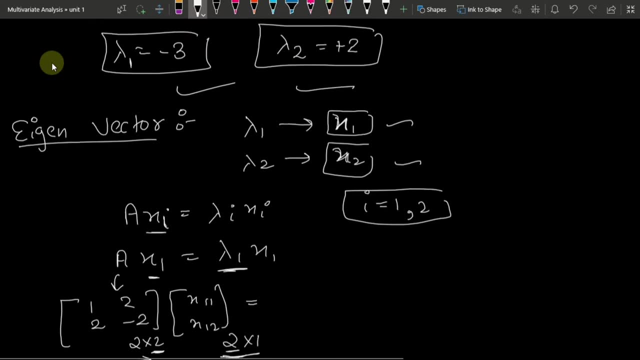 then we have to give 2 rows, then only multiplication is possible. so first of all, what is the value of lambda 1? we have the value of lambda 1, so we have 2 values. the value of lambda 1 is minus 3, so first of all we solve for minus 3. 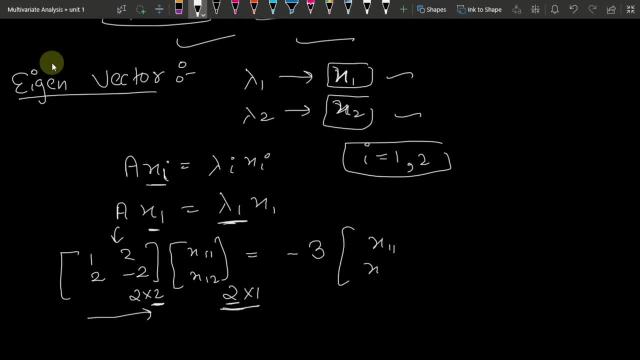 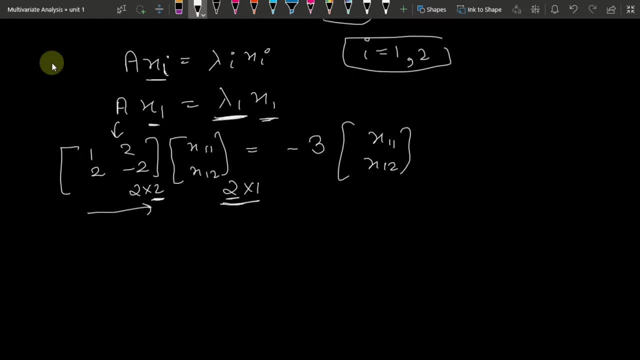 so minus 3, and here x1, 1, x1, 2, because after lambda 1 what we have to put is x1. so when we solve this we will have equations here plus 2, x1, 2, how it will be when you multiply the first row. 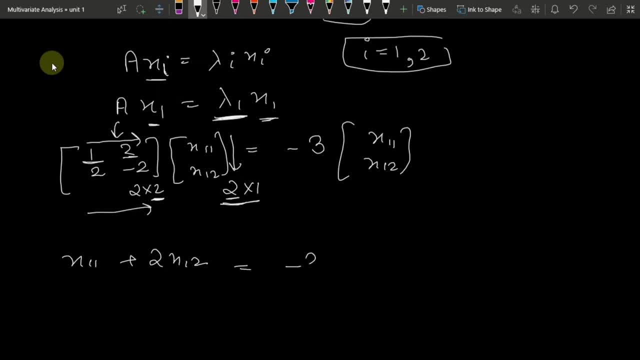 with this complete column. so x1 1 plus 2 x1 2 is equal to minus 3 x1 1, and second equation will be 2 x1 1 minus 2 x1 2 is equal to minus 3 x1 2. 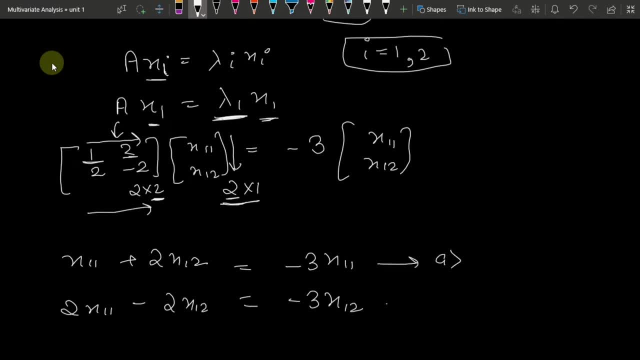 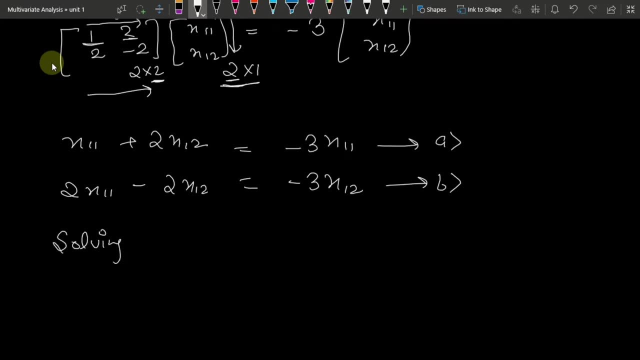 so when you mark these two equations, a and b, and when we solve them, what will we get solving a and b? when we solve a and b, we will get 4 x1 1 plus 2 x1 2 is equal to 0. we have put minus 3 x1 1. 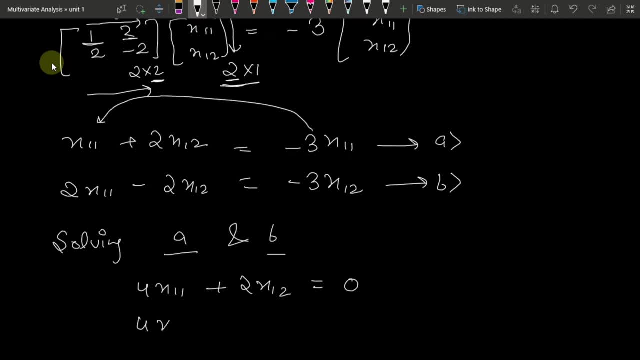 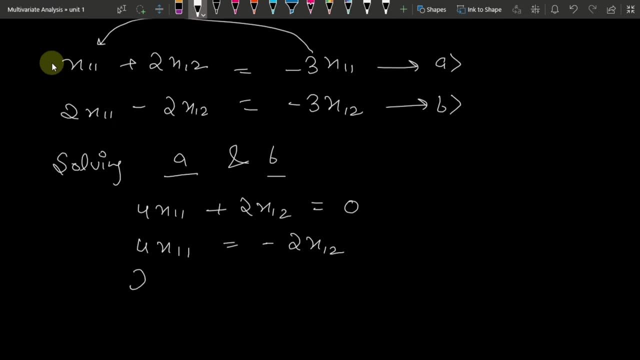 on this side. so what will we get? 4 x1 1 is equal to minus 2 x1 2. so this will be 2 x1 1 is equal to minus x1 2. so when you apply heat n trial method, so suppose, 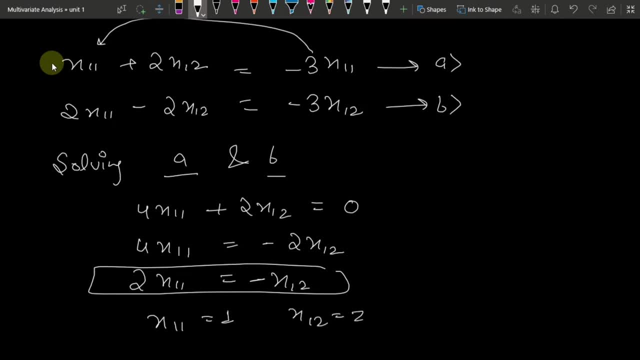 if you put 1 value of x1- 1, then how much will be x1, 2 minus 2? if you put 1 value of x1- 1, then how much will be x1, 2 minus 2? so your first eigenvector. 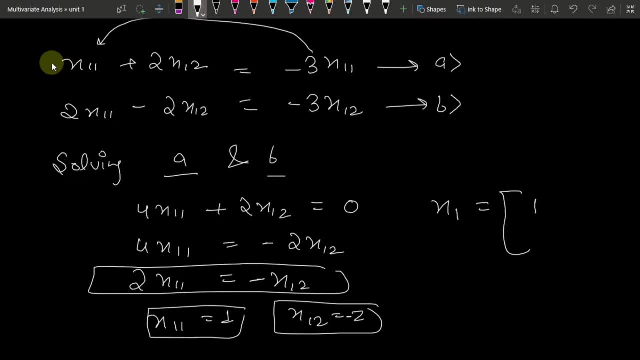 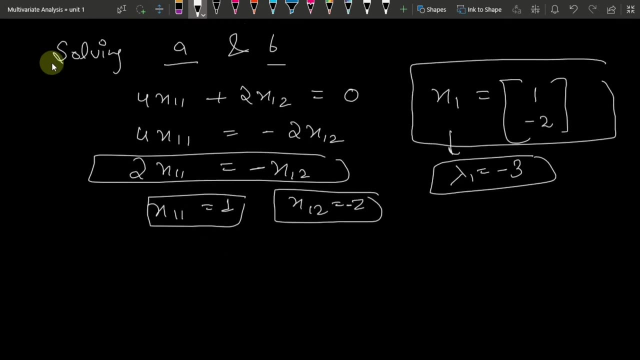 x1 is equal to 1 minus 2 and whose corresponding is equal to lambda 1. this is your first eigenvector. now from this you can also get normalized eigenvector. how to get e1: divide it by its length. what will be its length? 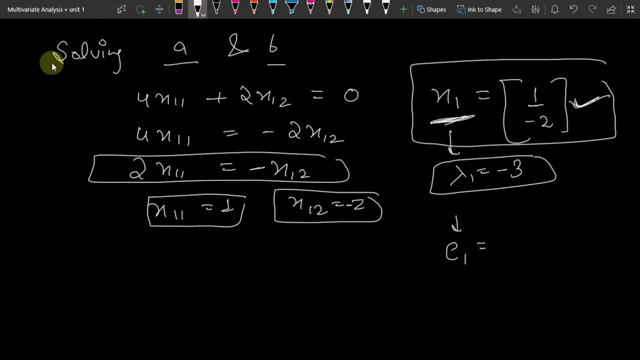 this is x1 vector. its length will be 1 square plus minus 2 square, so 1 square is 1 minus 2 square is 4. so what will be root 5? so here you have normalized eigenvector which you will use in your 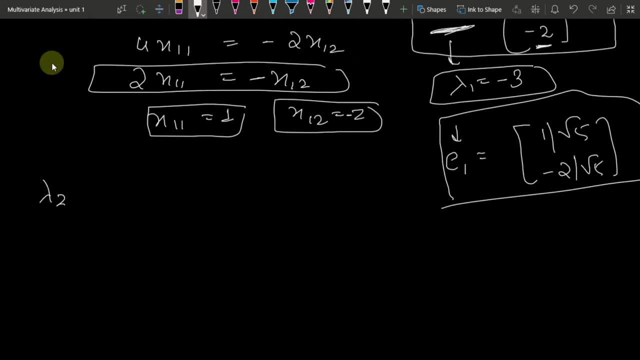 spectral decomposition. now for lambda 2. we have 2 for minus 3 we have taken. so again we will use a. x2 is equal to lambda 2, x2 because we are taking second. so what is a value of x2 and what is the value of x2? 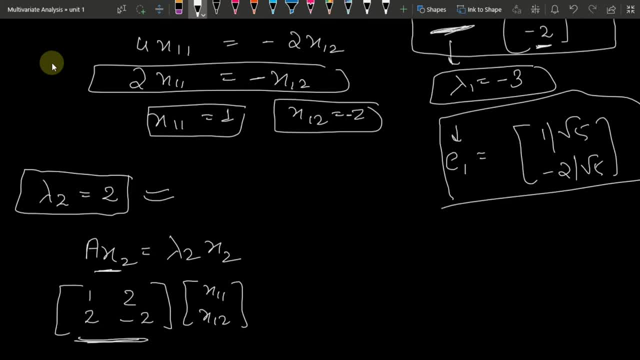 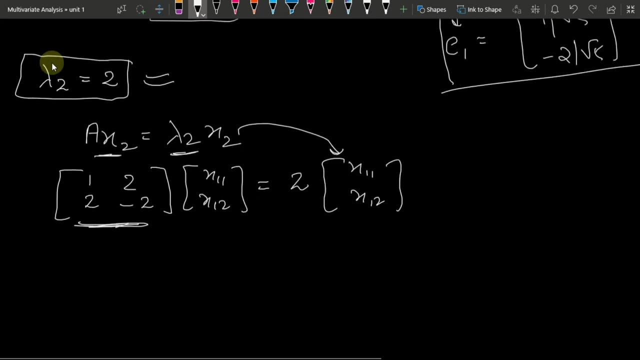 x1, 1. again we have to take vector x2 and vector will be taken according to its order. and lambda 2. we have put 2 and here x2, x1, 1, x1, 2. so what is x2 now when you solve? 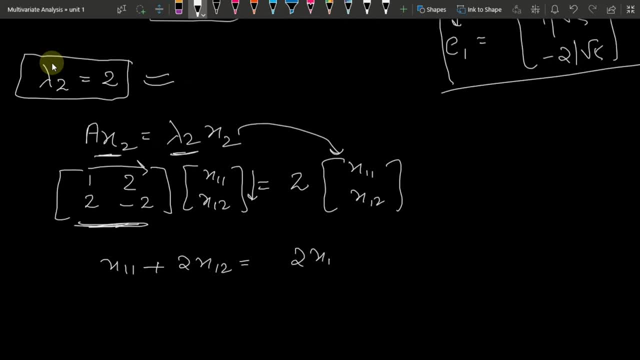 this equation, x1- 1 is equal to 2x1- 1. so when you subtract from here, a relation will come in x1- 1 and x1 2. that 2 times of x1- 2 is equal to x1 1. 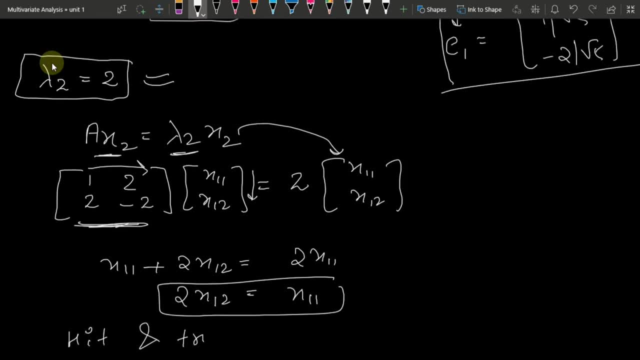 so when you apply possible values, heat and trial method, when we apply heat and trial method. so here we will make two equations but same relation will come from both. like we solved 1 if you put value of x1, 1 as 1. so if you put 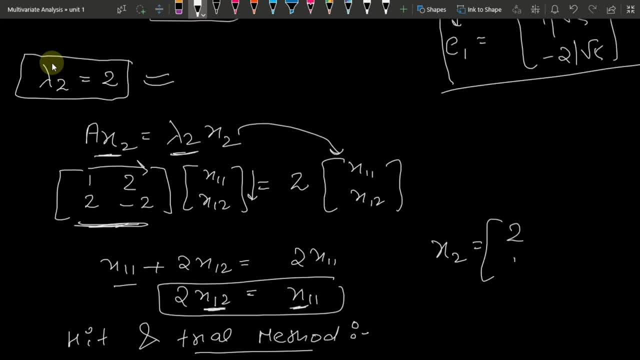 x1- 2 as 1, then x1- 1- 2 will come, so 2- 1. this way you will get a second eigenvector that is equal to x2. if you put x1- 2 as 1, then x1- 2 is equal to 2. 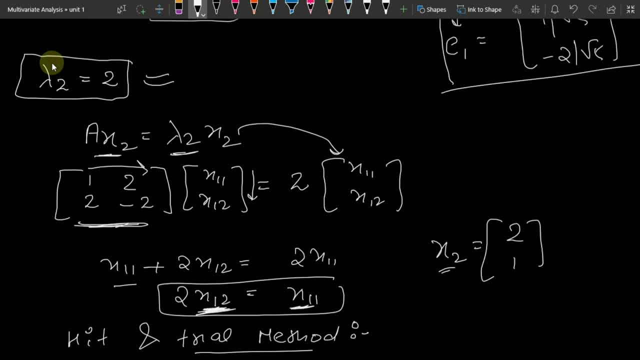 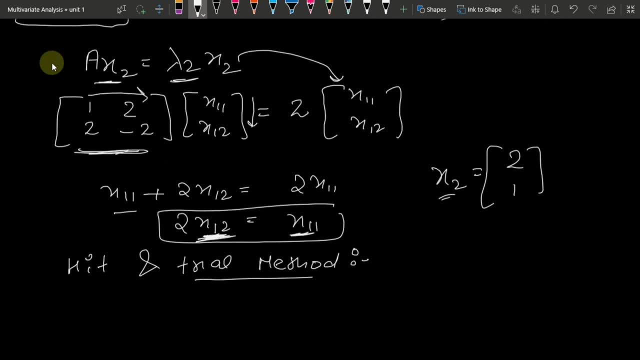 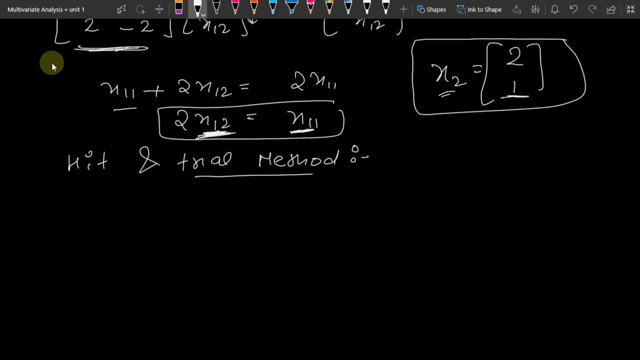 so here x1- 1 will come as 1. ok, so we put x1- 2 as 1. so x1- 1 is equal to 2. so this is second eigenvector. if you take out normalized eigenvector e2, then it will come. 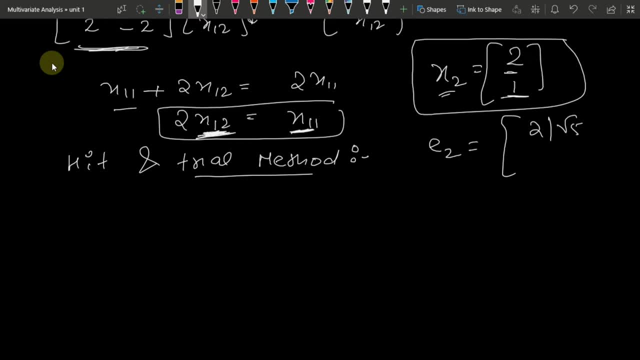 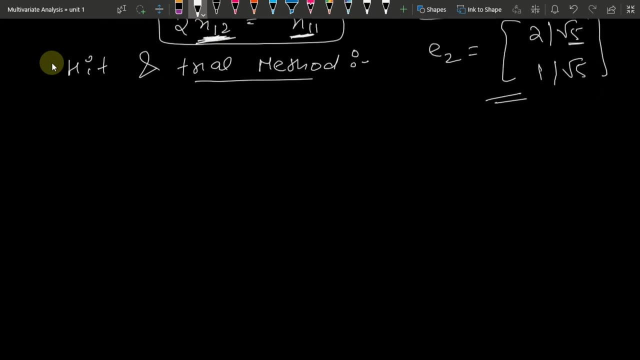 2 by root 5, because i divided it by length. length is 2 square 4 plus 1 square is 1 and root is 4 over 1 is 5, so this is normalized eigenvector. now we will do. we have found matrix eigenvalues. 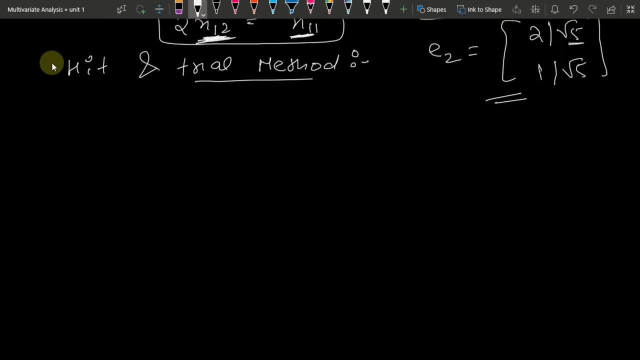 and eigenvectors. now we will prove the concept of spectral decomposition, that we can write any matrix in the form of eigenvalues and eigenvectors. so how? so what will be spectral decomposition if we write equation of spectral decomposition, spectral decomposition, spectral decomposition. so if we write: 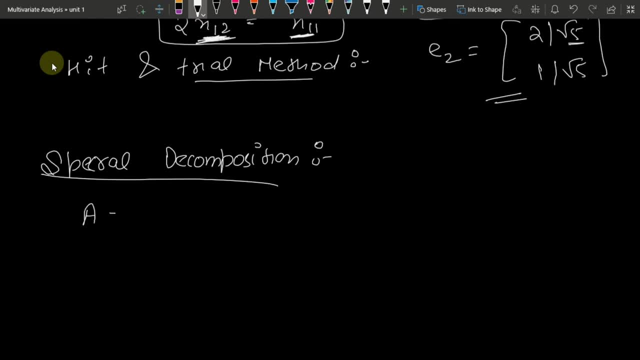 equation of this. so what was the equation? so you can write lambda1- e1- e1- transpose, plus lambda2- e2- e2- transpose. but will you write it further? no, because we have a matrix of 2 by 2 order, so it has only 2 eigenvectors. 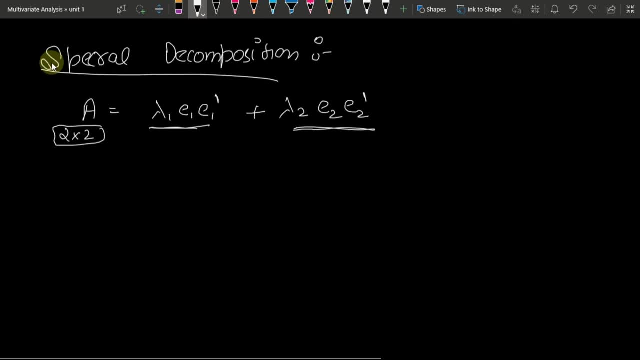 so we will keep it till here now. after this we will put values. we will take its right hand side, because right hand side we have to bring it equal to left hand side, that is equal to a. so we will take lambda1 e1, e1 transpose plus. 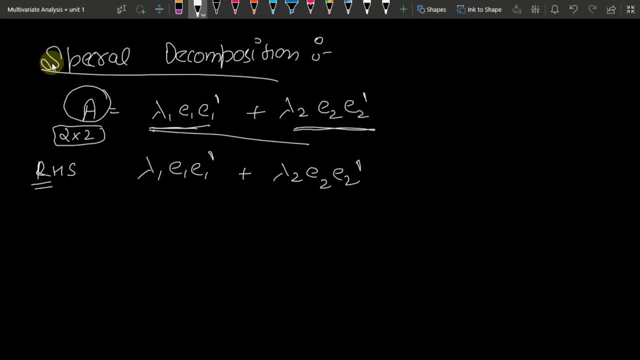 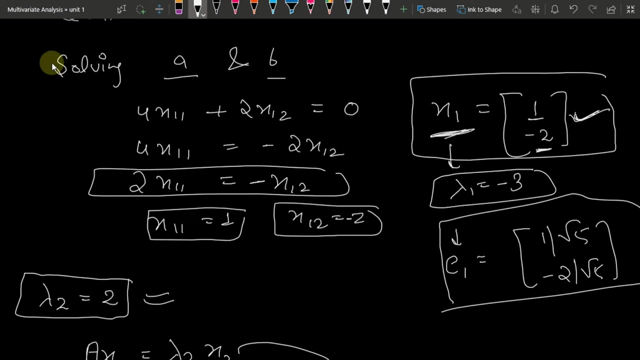 lambda2, e2, e2 transpose so lambda1. what was lambda1? we had minus 3 and what was e1? we had e1. now we will see we had e1 corresponding to e1, 1 by root 5 and minus 2 by root 5. 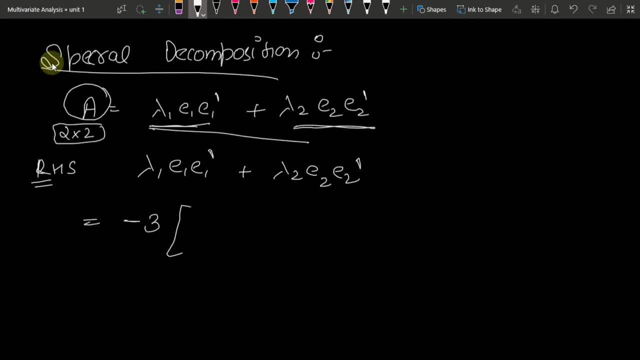 so 1 by root 5 and minus 2 by root 5. so we will put it and minus 2 by root 5, and after that what we have to do. e1 transpose means if we transpose it and write it horizontally, then it will be 1 by root 5 minus 2 by root 5. 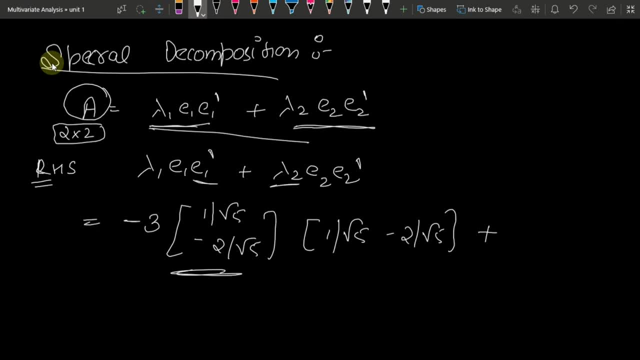 and after that, plus what was lambda2, we had 2, and what was e2? e2? we had just taken out 2 by root 5 and 1 by root 5, and if we transpose it then it will be 2 by root 5 and 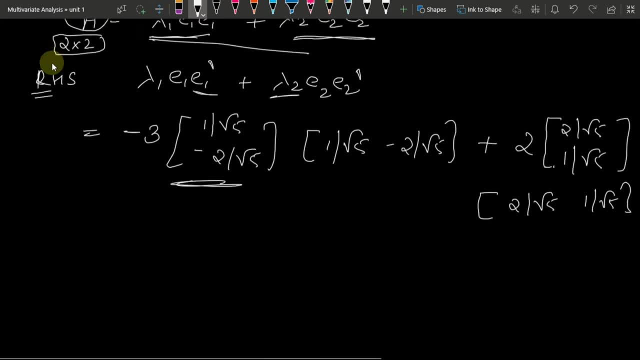 1 by root 5. so after this, when you solve it- so we know how to solve- we keep minus 3 as it is row by column multiplication, so this row will be from this column with first column. so this will be 1 by root 5. 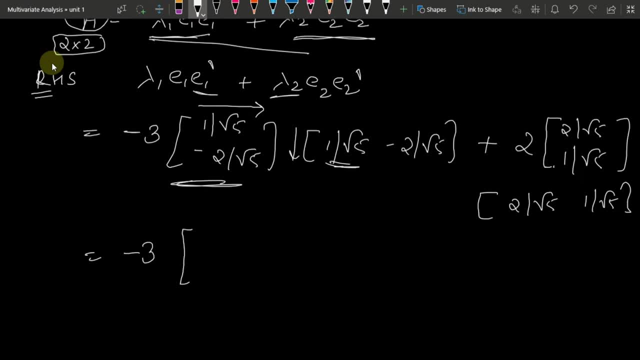 1 by root 5, so this will be 1 by 5. because root 5 multiply, root 5 will be 5. so this is 1 by 5. if you do it from next, 1 by root 5. if you do it from 2 by root 5. 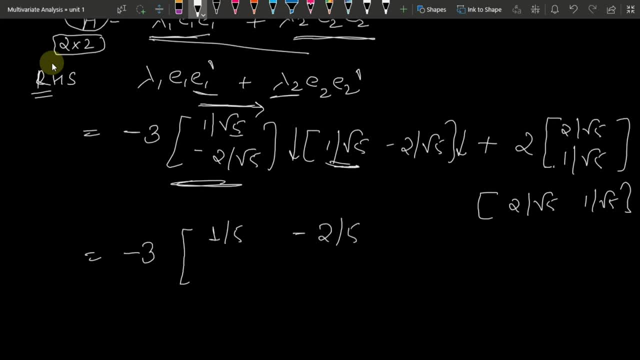 minus 2 by root 5, then it will be minus 2 by 5. why? because we have 1 by root 5 and root 5 will be 5, and if we do it from 1 by minus 2 then it will be minus 2. 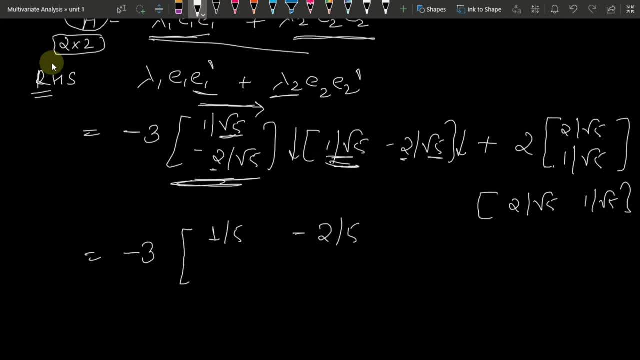 now we will do this element minus 2 by root 5 from 1 by root 5, so it will be minus 2 by 5. and if we do it with this 1 by root 5, then plus 2 as it is. and if you do now, 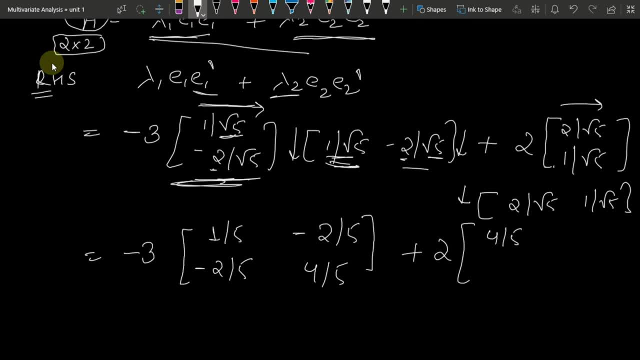 then this will come 4 by 5, and then with next, 2 by root 5. if you do this from 1 by root 5, then it will be 2 by 5, and then 2by 5, then it will be 1 by 5. 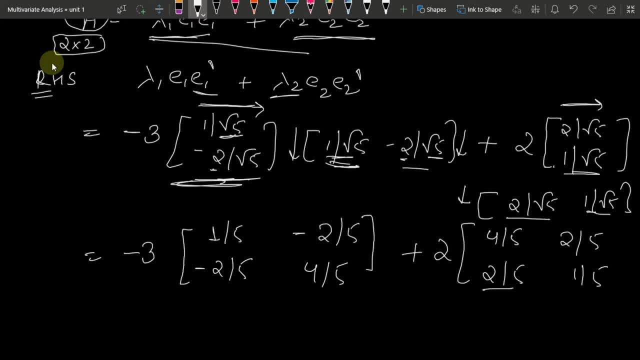 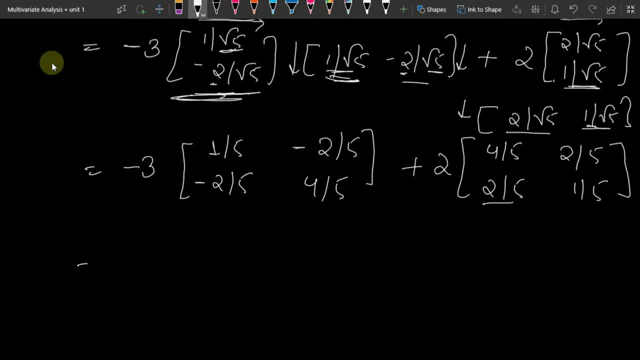 2 by root 5. 2 by 5. 1 by root 5. 1 root 5. now you have to solve. so this will be first matrix will be minus 3 by 5, multiply by minus 3, so this will be plus 6 by 5. 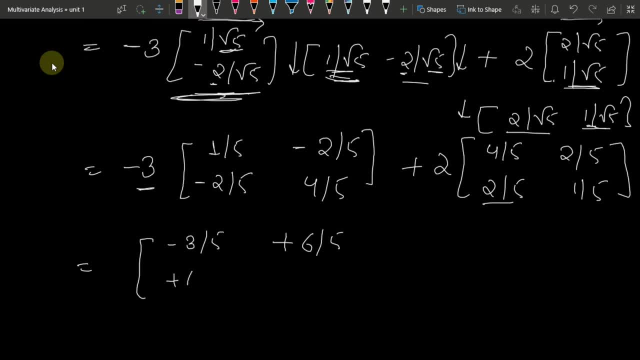 then this will be plus 6 by 5, then minus 12 by 5. why? because 3 is 4 and 12 is 5 plus 2. as it is, we multiply 2 inside, so we multiply 2 inside, so 2x4 is 8 by 5. 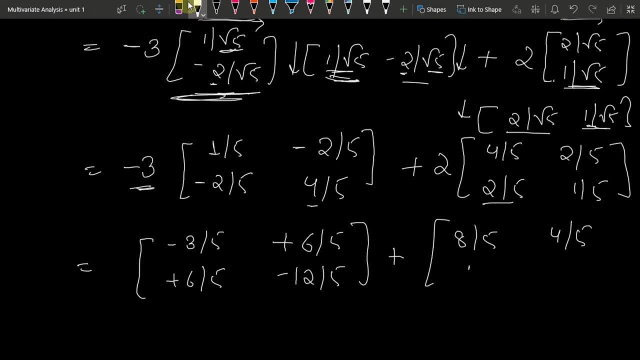 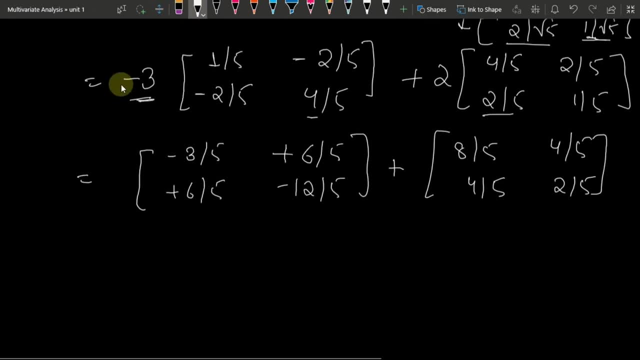 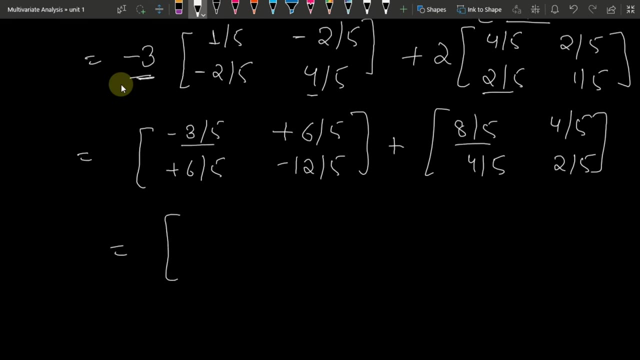 2x2 is 4 by 5, then 4 by 5 and 2 by 5. so we multiply inside now when you add both matrices. so what happens when we add? so when you add 8 by 5 in minus 3 by 5? 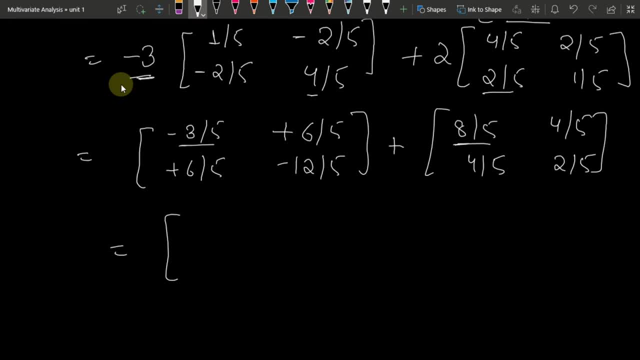 then LCM will remain 5 and 3 will remain from 8, because 1 is minus and 1 is plus, so 5 by 5 will be left, then 6 by 5 plus 4 by 5, so LCM will remain same: 5. 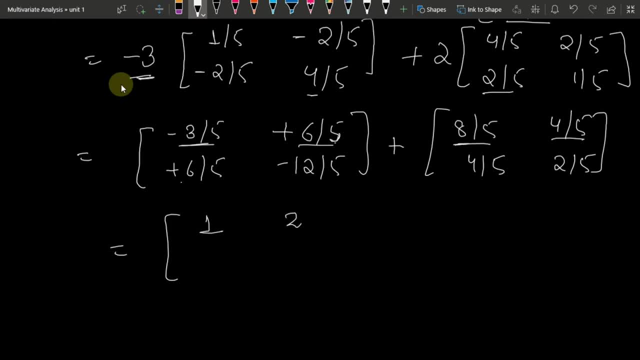 so 6 and 4 will be 10. so 10 by 5. this again 6 by 5. 4 by 5 will be same 2. then this minus 12 by 5 and plus 2 by 5. so this will be minus 10 by 5. 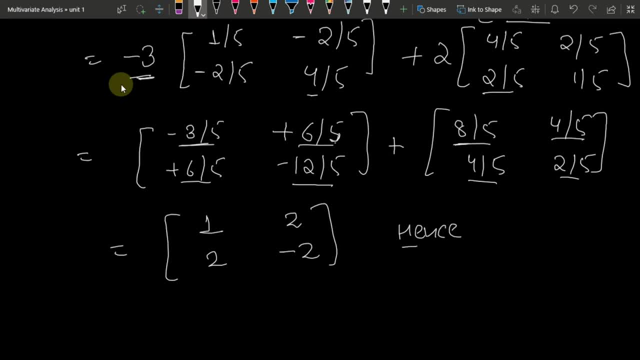 that is equal to minus 2, hence proved: we proved that we can write any matrix in the form of eigenvalues and eigenvectors. so what was this? the result was a- so you can check it: 1, 2, 2, minus 2. 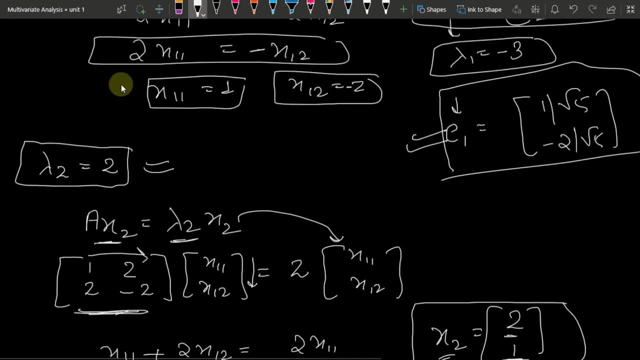 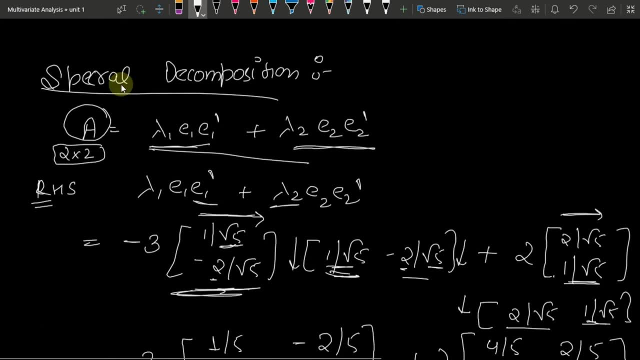 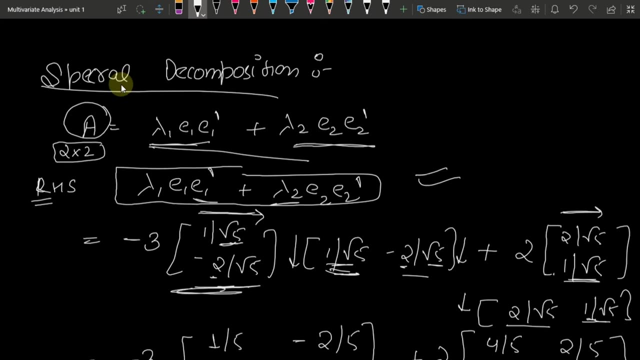 so let's check. so what was our matrix? this was our matrix: 1, 2, minus 2. ok, when we took this result, when we took right hand side, so we proved it of left hand side. so we can decompose any matrix in the form of eigenvalues and eigenvectors. 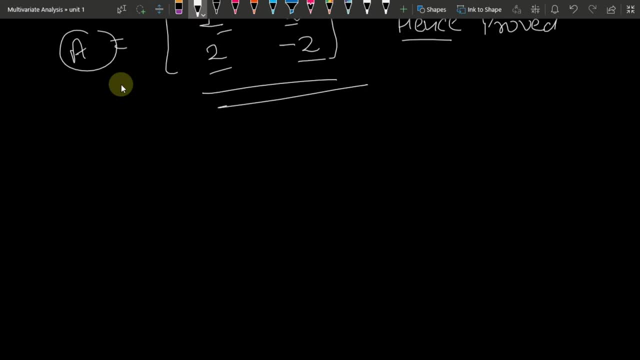 now, after this, we will see spectral decomposition in the form of matrix. so how we can represent spectral decomposition, so spectral decomposition in matrix form. so spectral decomposition in matrix form. so the spectral decomposition which we have done, we will write it in matrix form. ok, so how we will write it in matrix form. 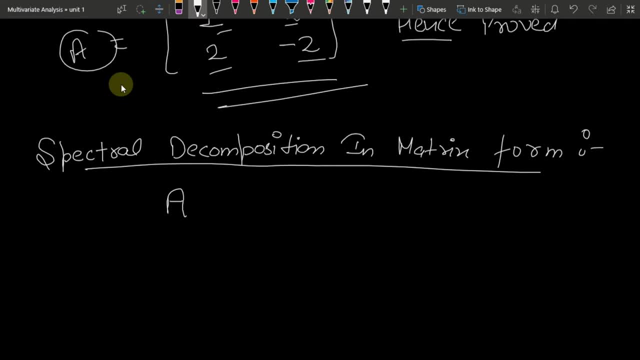 so if you had any one matrix, if you have any one matrix, square and symmetric condition- and it should be symmetric- then you can write it as O lambda, O transpose, O lambda, O transpose. now I will tell you that what is O, what is lambda and what is O transpose. 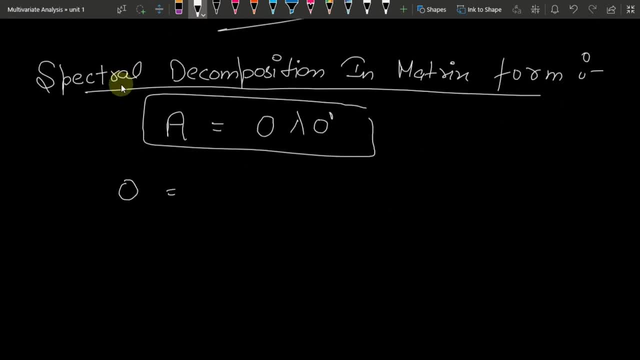 So here the O will be. this will be a vector of normalized eigenvectors. okay, so this will be. we have E1, E2, E3, up to which we have normalize eigenvectors of E, their one, their matrix, or we say their one vector. okay, and the lambda will be diagonal matrix. 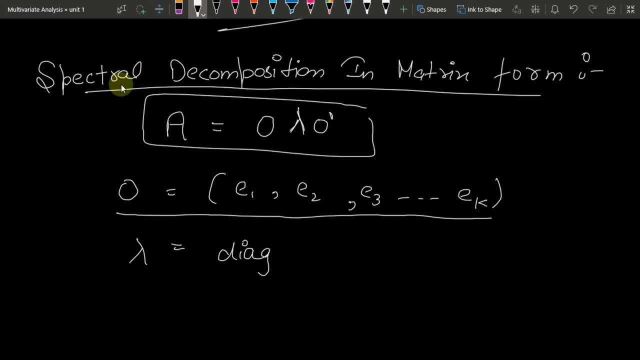 what will be lambda, a diagonal matrix. so here the lambda is showing this will be a diagonal matrix of all eigenvalues. so you can write it like this: that the lambda will. so it will be like this: lambda1 0 0 0. 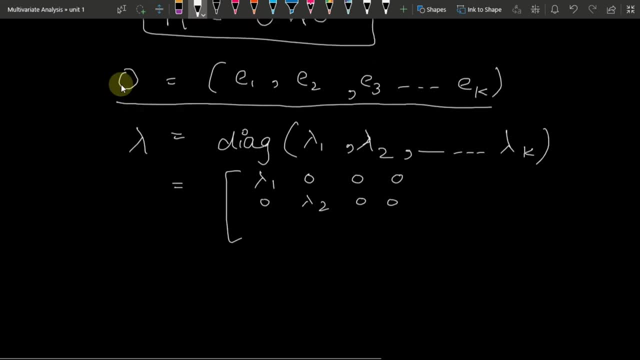 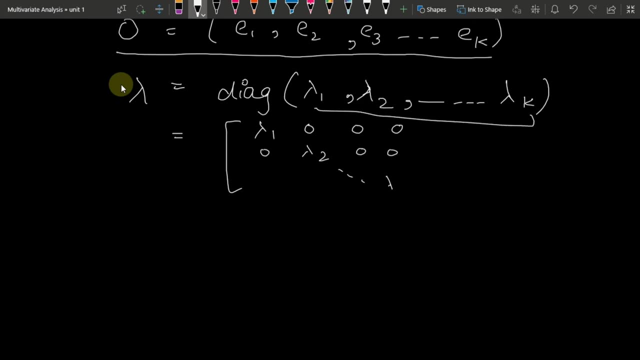 then 0, lambda2, 0, 0, 0. so this is diagonal matrix. what is diagonal matrix in which diagonal elements will be lambda1, lambda2, lambda k, but other elements will be 0, so other elements will be 0. so in this way you will have lambda. 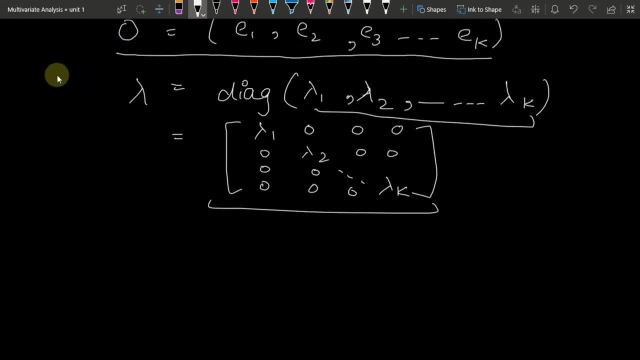 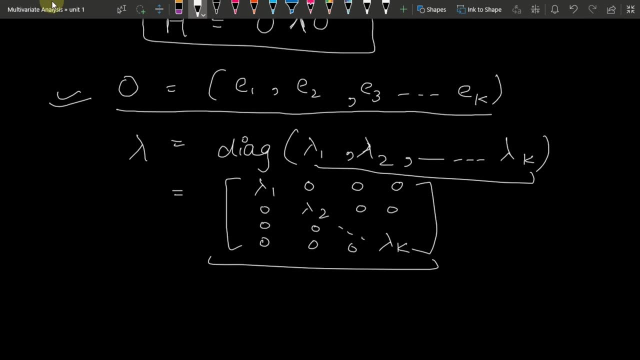 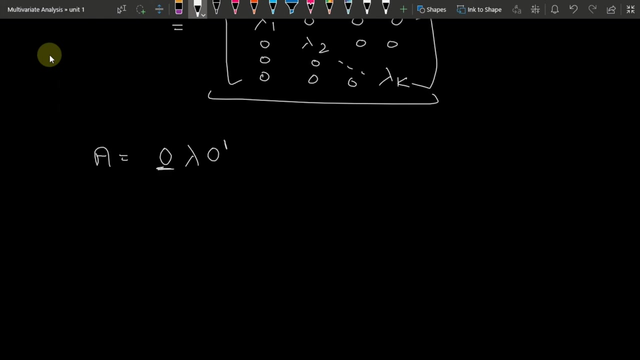 and O. O will be the matrix of normalized eigenvectors. ok, so now when we solve this, like in the previous example, in the previous example we can write A in the form of O, lambda O transpose. so what will be O? what will be O? then we said that O will be. 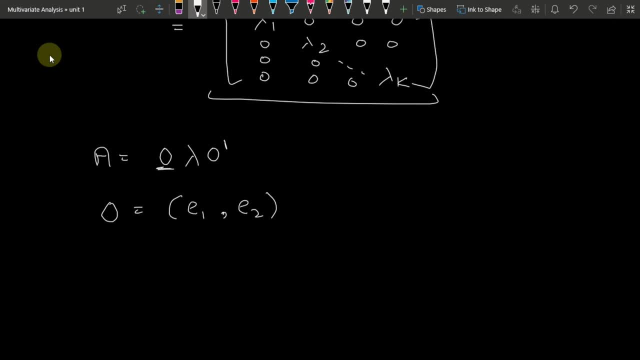 E1 comma E2. so because we had A, which was 2 by 2 order matrix in which we did example, so it had only 2 eigenvectors. and what were those normalized eigenvectors? 1 by 5, 1 by root, 5. 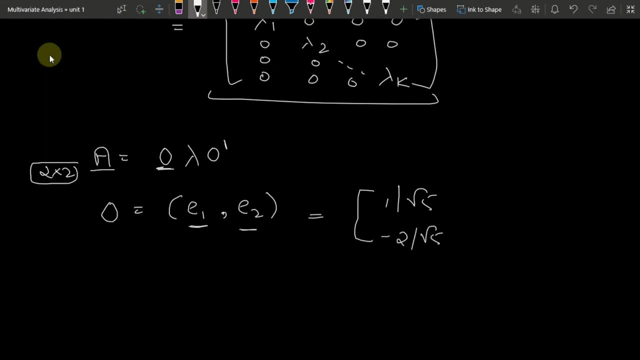 and minus 2 by root 5 first. was this? so first you have to write as it is in a column, means E1, you have written in this way in a column, and second, the E2 as it is, you will write it in the form of a column. 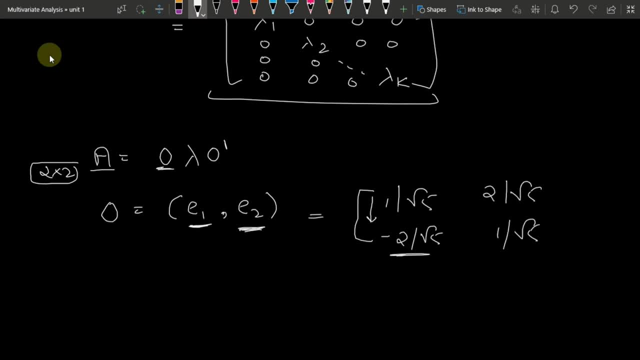 2 by root 5 and 1 by root 5, so you will have O matrix means eigen matrix of normalized eigenvectors. if you will transpose it, then how to transpose that? your row will be a column, so 1 by root 5, 1 by root 5. 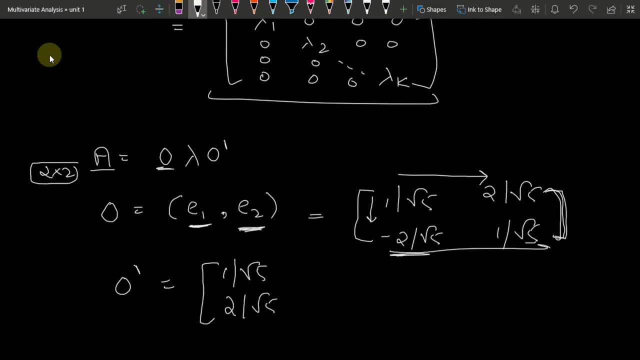 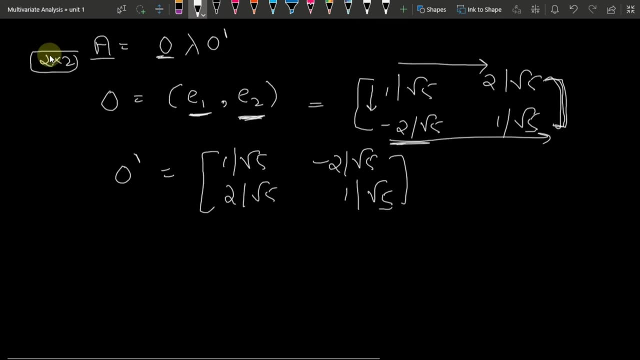 2 by root 5 and in the same way, this row will be the next column. so minus 2 by root 5 and 1 by root 5. so you now the matrix A. you can construct it again. O lambda, O transpose, and what will be lambda? 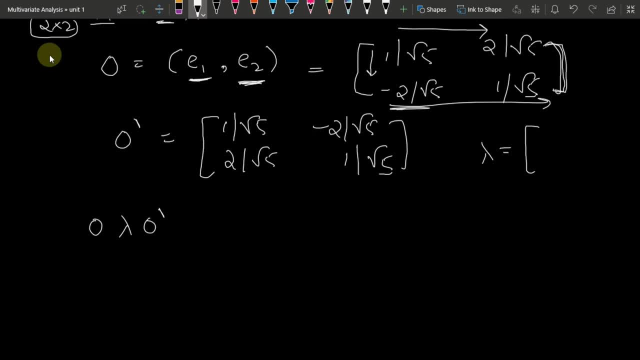 lambda is left. so what will be lambda? what was the first eigenvalue we had first, ie lambda: 1 0 0. lambda will be like this. so what was the first eigenvalue? you had minus 3. what was the first eigenvalue you had written? 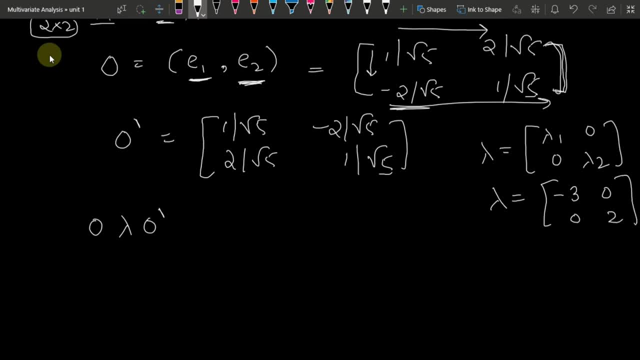 minus 3, 0, 0 and second 2, so you will write it like this: what was O? we just had 1 by root 5, 2 by root 5, then minus 2 by root 5 and 1 by root 5. 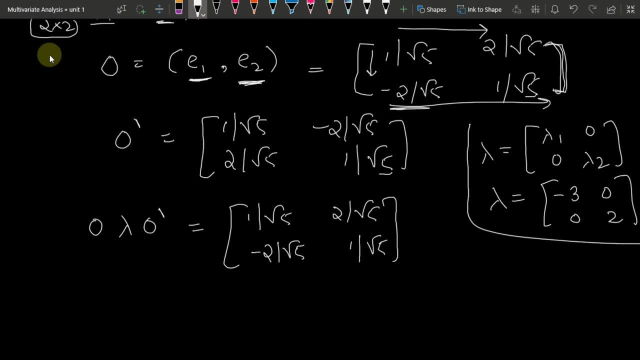 so this: ok, we have written O, then lambda, what we have minus 3, 0, 0, 2 and after this O transpose. so what is that? 1 by root 5 and 2 by root 5 and 1 by root 5. if you solve it again, 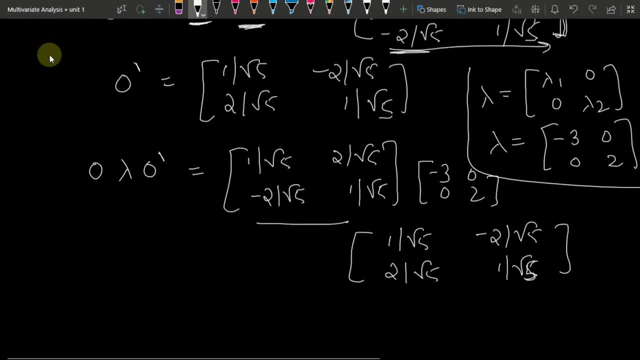 if you solve it again, then you will get same result, ie the same what we have just proved, the same proof this is, but in which form? matrix form. there we were writing eigenvalue and eigenvector individually, as we did here, what we did here. 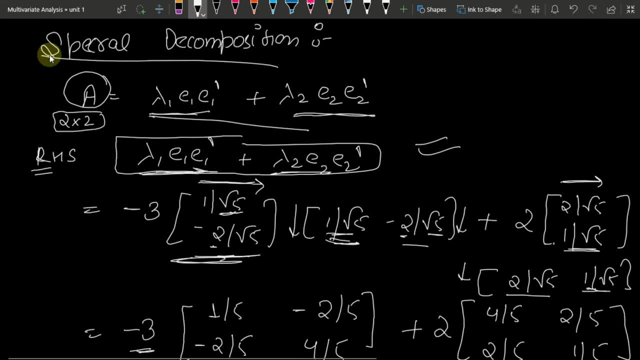 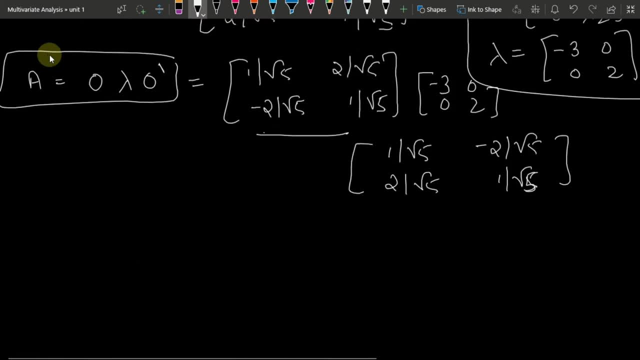 that every eigenvalue and eigenvector product was written individually, but here we write it in a matrix form. ok, so when you do its product and when you do its product, so you will get 2 by 2 order matrix and that 2 by 2 order matrix. 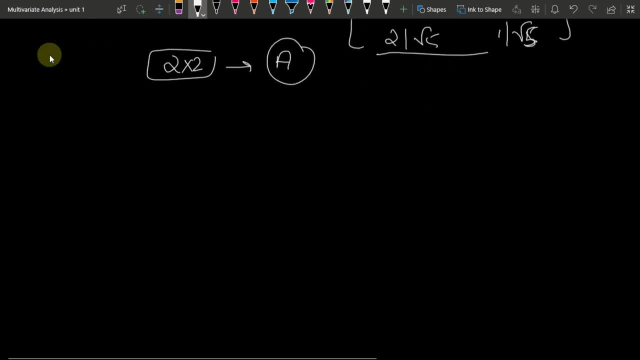 will be A which you solve. so now, some properties are there, what other properties are there? so if we see first property of spectral decomposition here, so if you have any other positive definite matrix, so property we are seeing here, that then a for a positive definite matrix. do we know? 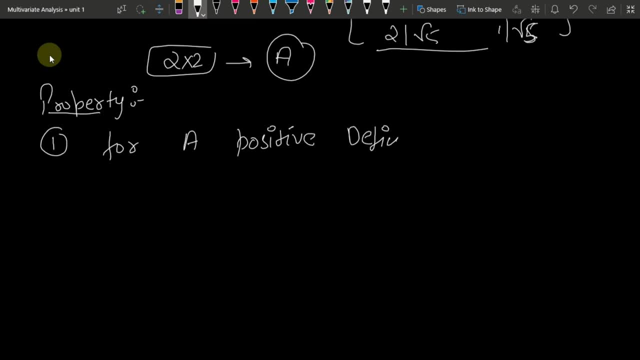 what are the positive definite matrix, whose eigenvalues, some are positive for the positive definite matrix. so, for a positive definite matrix, and we thought that the positive definite matrix is one, so now brave own eigenvalues, μας eigenvectors. you can also find inwards of. 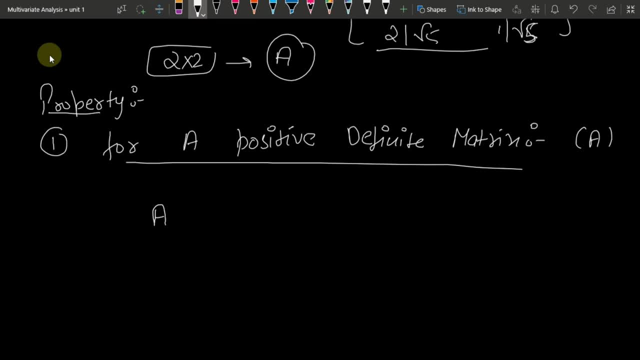 any matrix like till now. you have used eigenvalues, eigenvectors and found that matrix. you can also find out the inverse of matrix, like: A inverse is equal to O. what will be the difference? like for A: A is equal to O, lambda O transpose. if you take out A inverse, 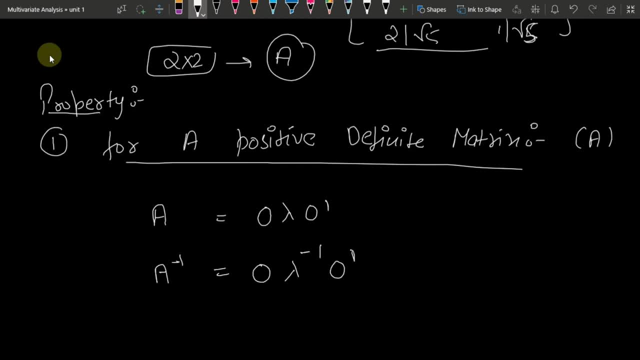 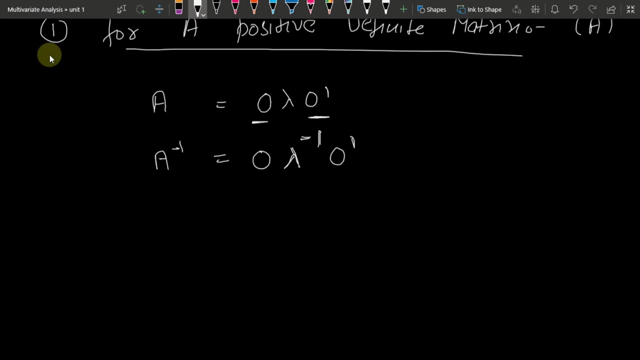 then it will be O, lambda inverse, O transpose, O and O transpose will not have any effect on matrix sign, only lambda will be inverse. so what will be the inverse of lambda like? we took out lambda matrix like minus 3 0, 0, 2. so here you have to use lambda inverse. 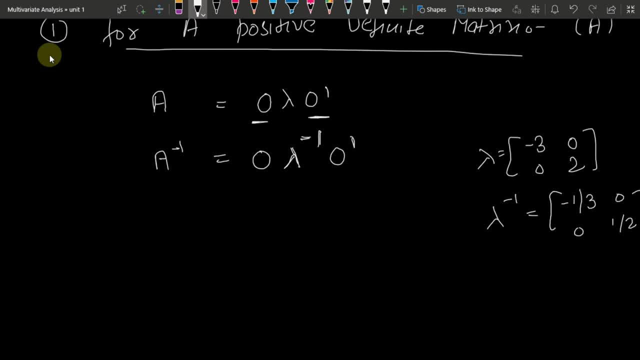 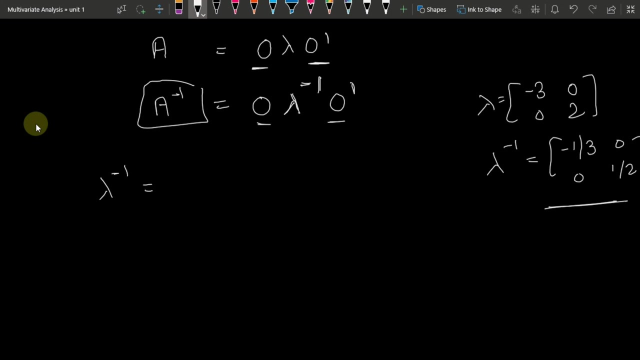 like minus 1 by 3, 0, 0, 1 by 2, like this. and O and O transpose will be same. so you can find out the inverse of any matrix. so we can write: lambda inverse will be a diagonal matrix in which diagonal elements will be 1 by lambda 1. 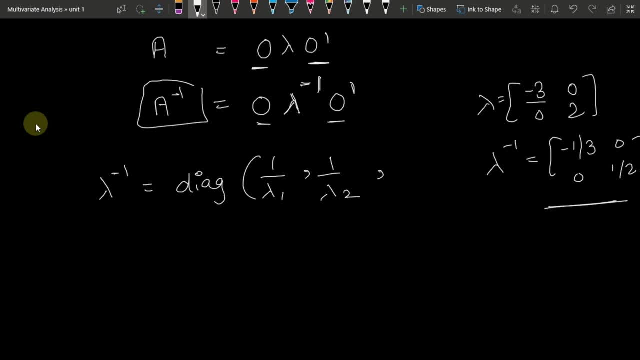 1 by lambda. 2, like minus 3, is equal to minus 1 by 3, 2 is equal to 1 by 2, so you can find out the inverse of lambda matrix like this and I have told you how to find out O and O dash. 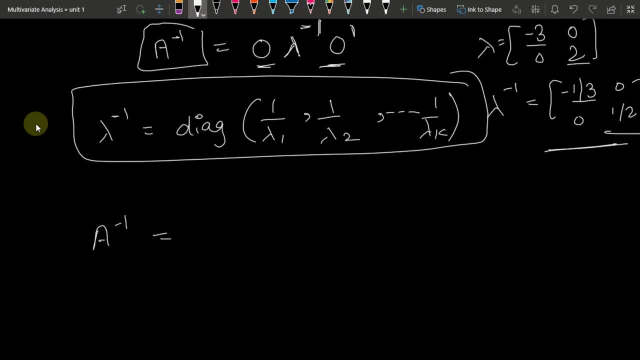 so we will write it in other form. like A inverse is equal to, so it will be J, equal to from 1 to K and 1 by like for simple. what was it lambda I, EI, EI transpose here it will be 1 by lambda J, EJ, EJ, transpose. 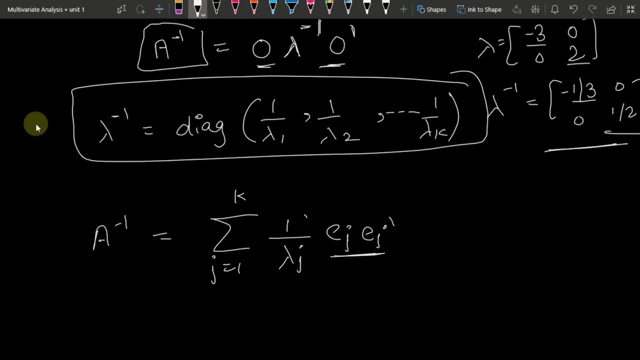 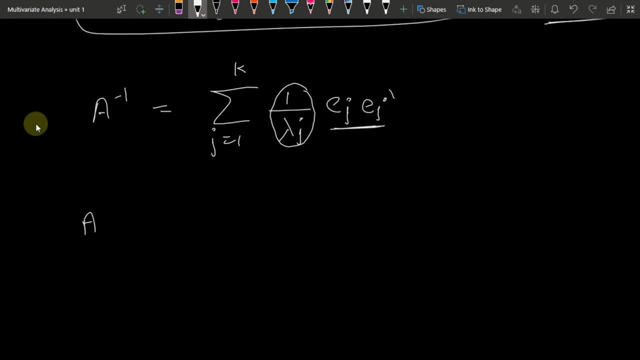 means these vectors. there will be no effect on them, only their eigen values will be reversed. similarly, if you want to find out the root of any matrix like this, then you have to find out the root of any matrix like this. so it will be O lambda power 1 by 2. 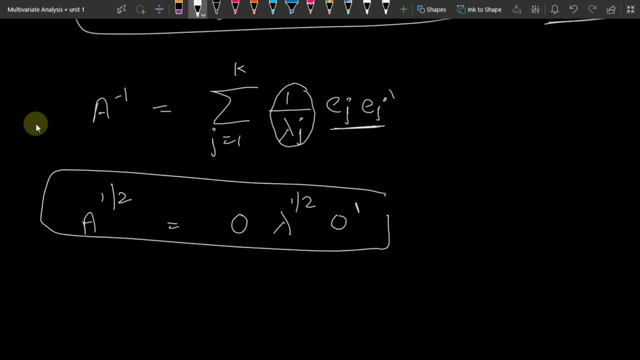 O dash. so it will be the same O and O dash. you have lambda. its power will be changed. if you want to find out the inverse of A, then it will be lambda inverse. if you want to find out the root of A, then it will be. what will be the root of lambda? 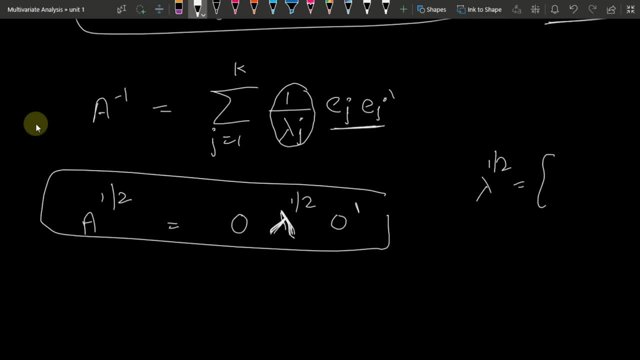 like: let's take again what will be the power of lambda 1 by 2, like here: we have root of minus 3, so its root will be root minus 3, 0, 0 and root 2, so you can find out like this: ok. 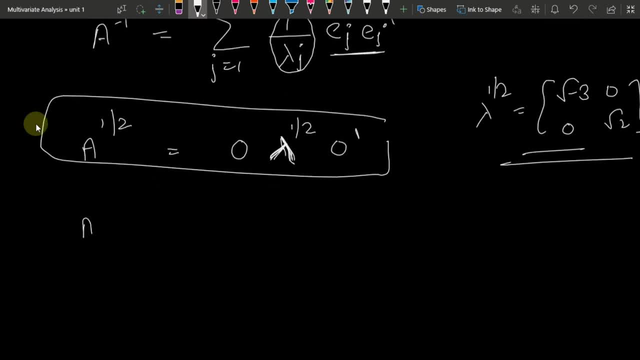 so if you write it like this: A power 1 by 2, this is matrix form. this is matrix form. so from here you will get summation J equal to 1 to K under the root, what will be the root of lambda J and EI. EI transpose will be same.